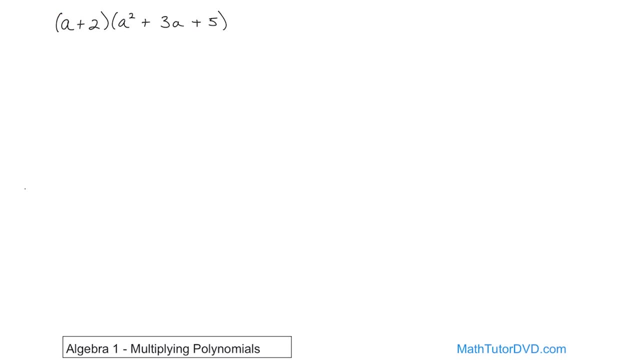 wasn't even there. so there was two terms in here. you already know how to do that. You take a times this and a times that, And then you go here and you do two times this and two times that. But now you have a third term. So what do you think you do? Well, what? 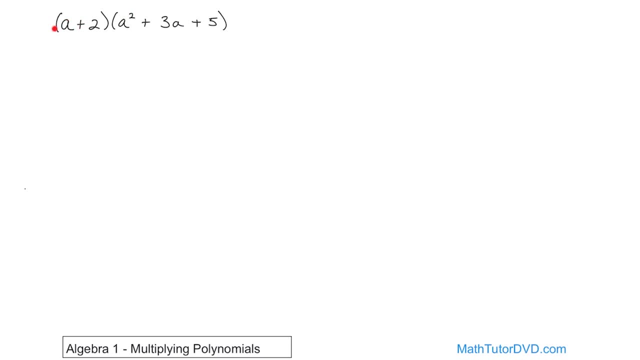 you do is you start with this first term, multiply this times that term, And then you go here, then a times the three a, Then you have to distribute the a times the five, So it gets distributed into all three of these terms. Then you move over to two, You distribute. 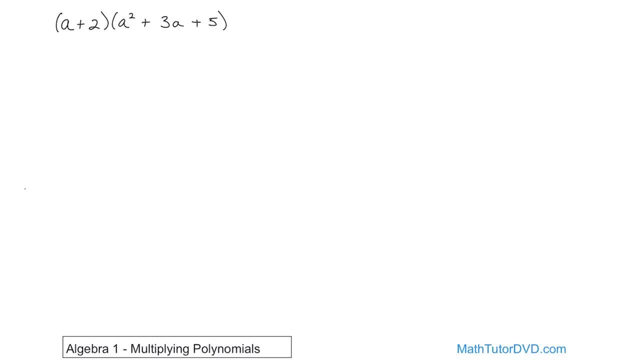 them here. you distribute them here. you distribute them here. And that's the blueprint for how you multiply any two polynomials together. Every term you have on the outside gets multiplied times every term in the second polynomial. Then you move to the next term and you do. 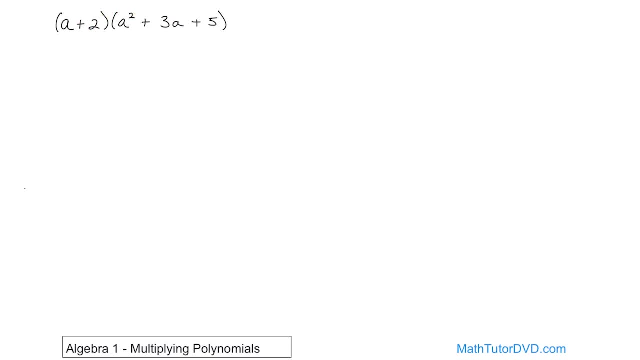 exactly the same thing. And then you keep doing it until you've multiplied everything together and then you simplify terms. So this case, for instance, we have a times a squared is going to give you a cubed because we add the exponents together. Now we take the a times the three, a It's going to give. 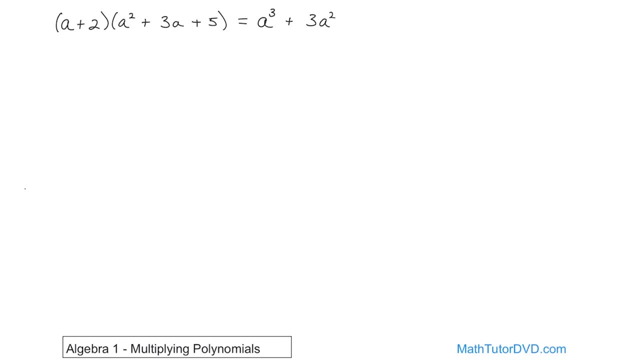 you three a squared, because we add the exponents together, one plus one. Then a times five is five a. So we're done with this guy up here. Now we move and turn our attention to the positive. two times the a squared gives us two. 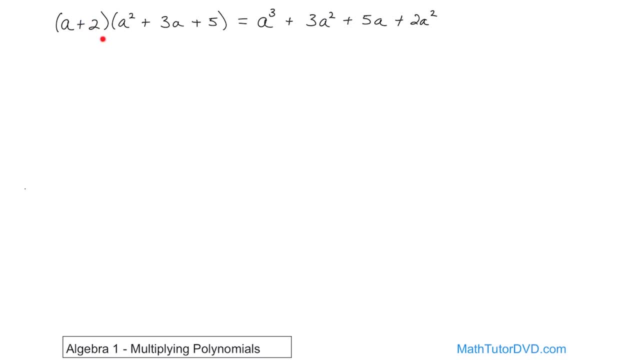 A squared. Then we take the two, multiply it times the three, a. So two times three is six, a. All right. Then we take the two and multiply it times the five. Two times five is ten. So you see how that works. We're just multiplying everything on the outside times. 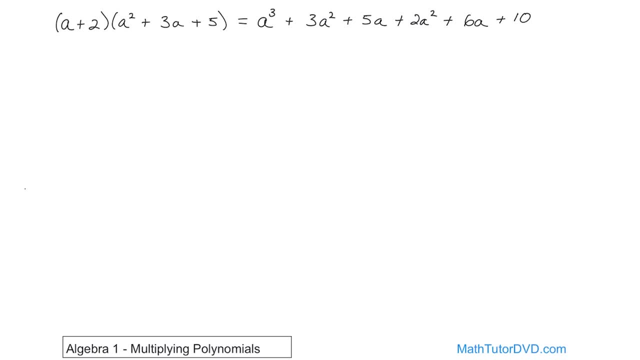 everything on the inside. Now we look for like terms. So we have an a cubed. We don't have any more a cubed, so we don't have anything else to add him with. But we do have an a squared And we can add him to that a squared. So we do have an a squared And we can add. 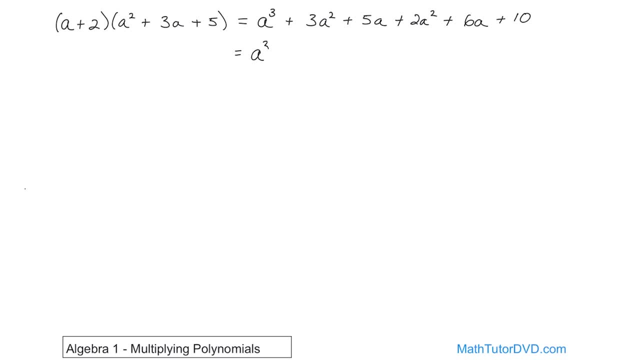 him to that a squared. So let's go ahead and mark that down. First we have the a cubed, That didn't change. Then we have three a squared and two a squared. Three plus two is five, So five a squared. Now we have five a and six a. Those are like terms and together they 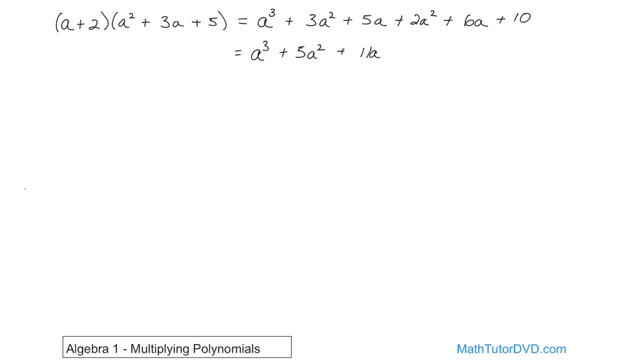 make eleven a, And then we just have one constant. There are no other numbers here. so you have plus ten. So the answer is a cubed plus five, a squared plus eleven, a plus ten. That's the final answer. Now let's see why we're naming this section multiplying polynomials, Because here I have. 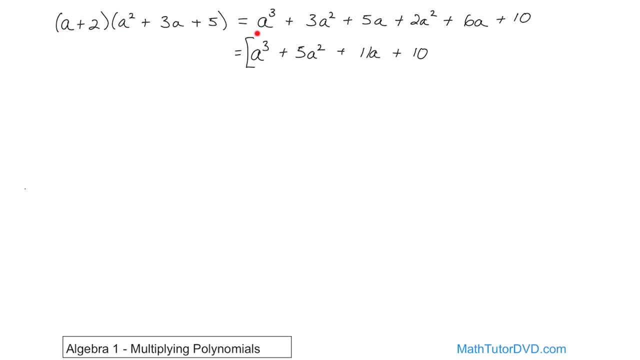 two terms times three terms. But I could have two terms times four terms. If I had a fourth term in here, then a would just get distributed to everything, including that fourth term before I move here going four terms. So it's the same general pattern. You can multiply any. 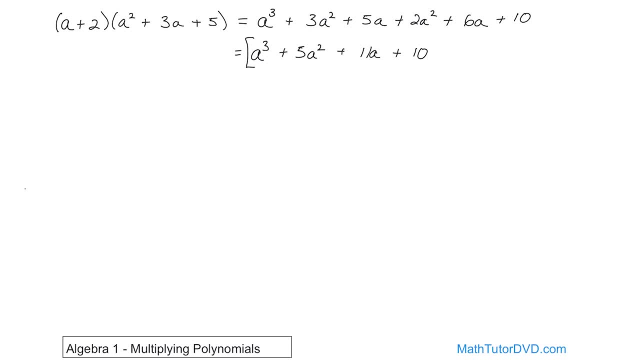 two polynomials together using this technique. And now you know why I don't really like the idea of teaching FOIL- The word FOIL, Because it teaches you to remember those letters rather than what you're doing, If you know what you're doing, which is just distributing these terms. 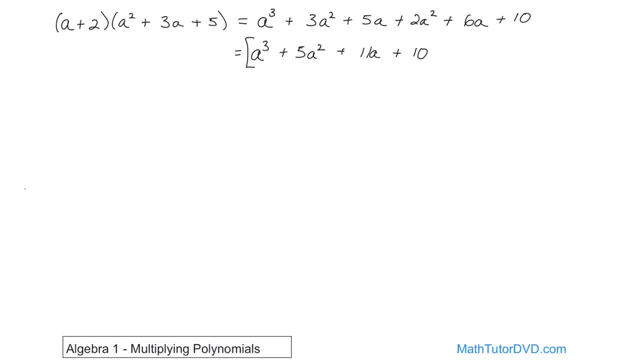 in. then you can multiply any two polynomials. You don't have to remember any rules, Alright. so the next question is going to be: now that we know what we're doing, we'll just start cranking along here. What if we have two x minus, one times x squared minus x plus? 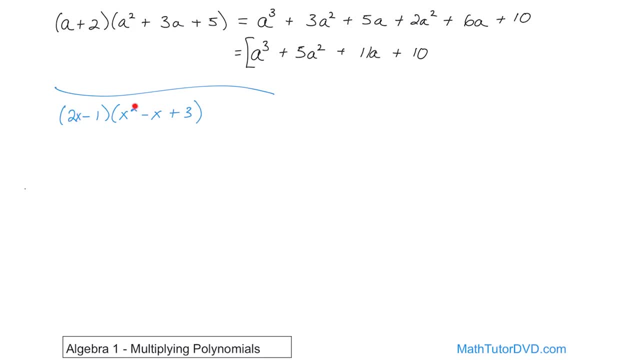 three. So we start here. Two x times x squared gives us two x cubed, because we add the exponents. And then two x times negative x. Don't forget, the negative is negative. two x squared Because we add those exponents. Then two x times three gives us six x. Now we're done with distributing. 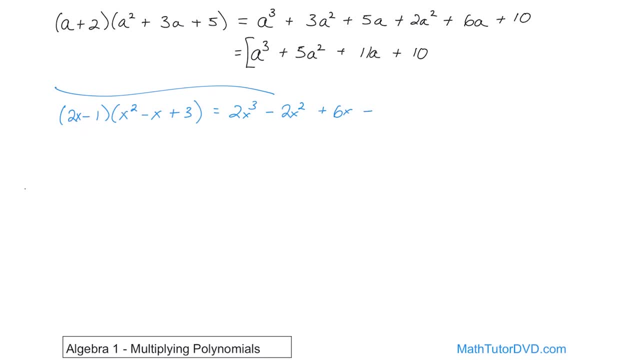 this in. Now we look at the negative. one times the x squared gives you negative x squared. Then we have the negative. one times the negative: x gives you positive, x Negative times. negative gives you positive gives us negative. 3. Now we look to collect like terms. We don't have any more x cubes anywhere. 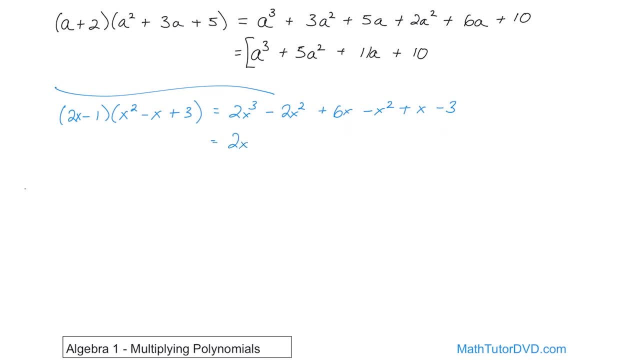 here. so we can't really do anything with that. We just write it down: 2x cubed. We have negative 2x squared and negative 1x squared, which is going to give us negative 3x squared. Then we have 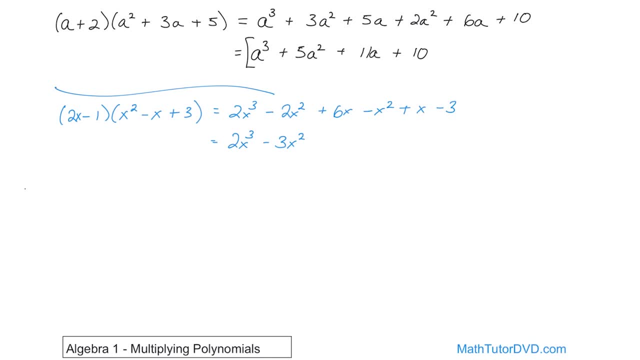 positive 6x and positive 1x, which is going to give us positive 7x, and then we have the number negative 3. there There's nothing left to add him to. So what we have is 2x cubed minus 3x squared. 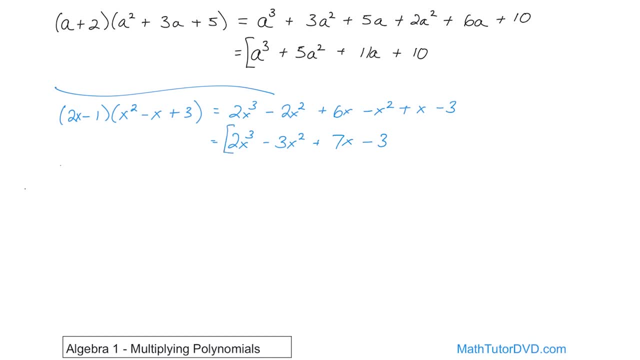 plus 7x minus 3.. That is the final answer, right? So once you get the idea, once you get the hang of it, it's not that hard. okay, Let's try another one. Let's say we have 3z minus 2 times 3z. 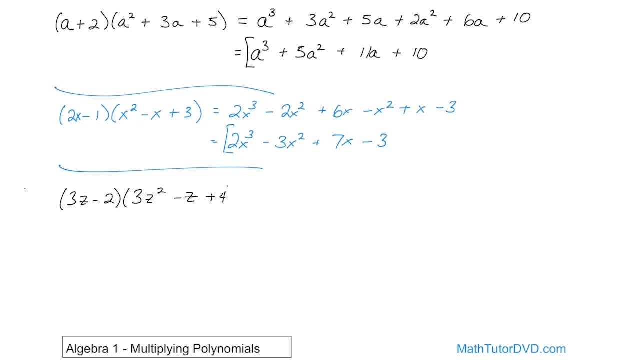 squared minus z plus 4, and we want to multiply all this together. So we start with the 3z times: 3z squared minus z plus 4, and we want to multiply all this together. So we start with 3z. 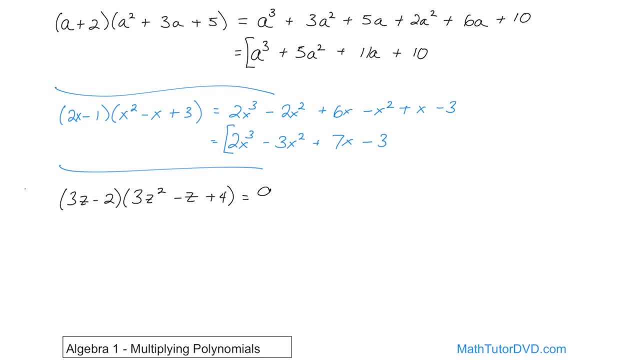 times 3z, squared minus z plus 4, and we want to multiply all this together. So we start with 3z times 3z. squared 3 times 3 is going to give you 9.. z times z squared is going to give you z. 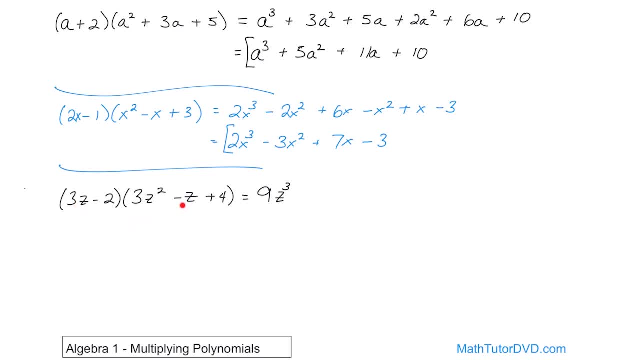 cubed. We add the exponents. Then we take this times negative z. It's going to give you negative 3z, squared, because we add the exponents. Then we take this times positive 4.. It's going to give you 12.. 3 times 4 is 12z. Now we're done with this. Now we turn our attention to negative 2. 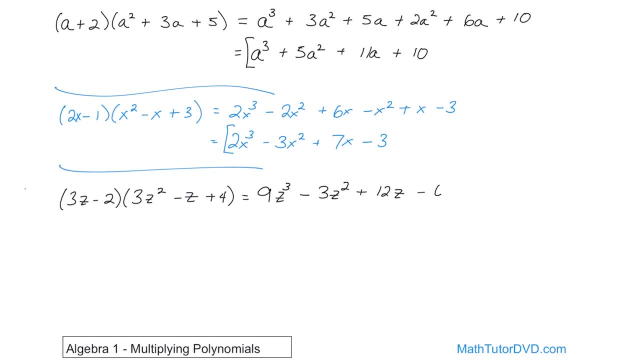 times 3z squared, It's going to give you negative 6.. z squared, And then we have negative 2 times negative. z is going to give you positive 2z. Then we have negative 2 times positive. 4 is going to give you negative 8, like this, Okay. 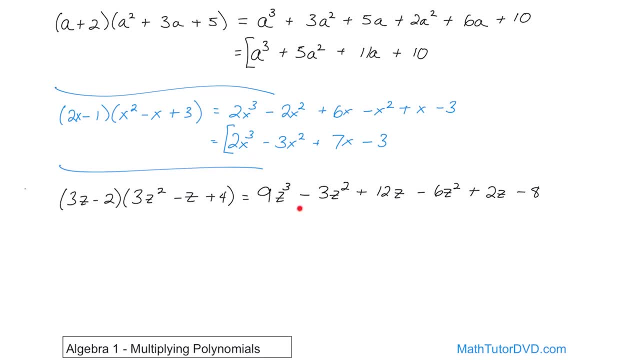 So now we look at like terms, We don't have any z cubed other than that initial one. So what we have is we write it down: 9z cubed. Then we have negative 3z squared, negative 6z squared. We add: 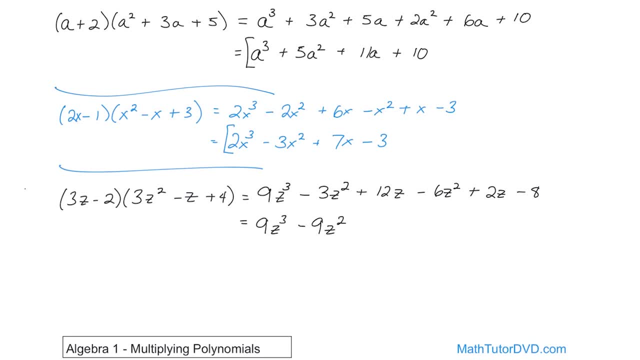 those together and we get negative 9z squared. Then we have 12z and 2z. We add those together, We get 14z, And then finally, we have negative 8.. There's nothing to add there, So we get 9z. 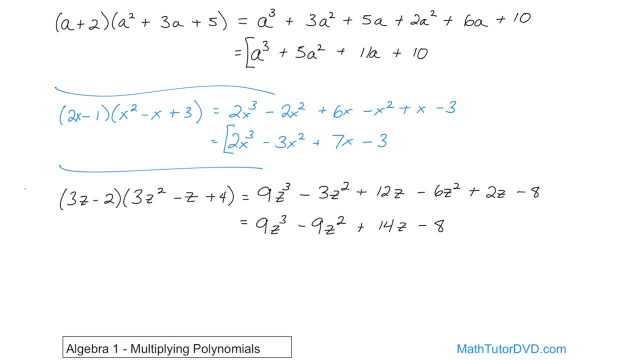 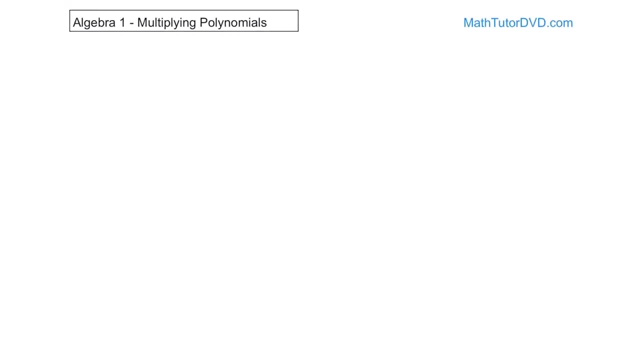 cubed minus 9z, squared plus 14z minus 8.. That is the final answer. All right, Just want to do a couple more to let you get some practice. So we're going to shift up And by all means pause the video. See if you can solve them yourself. I mean, that's the whole point. 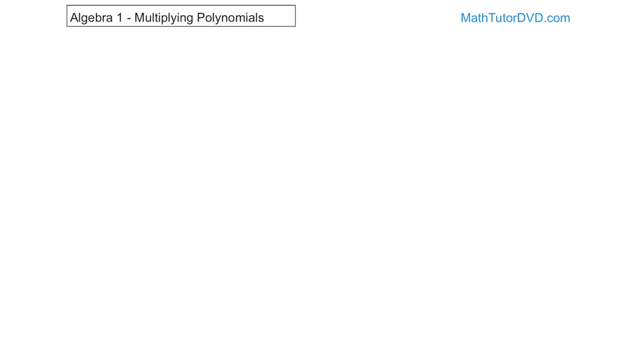 to see if you can do it on your own. And none of these problems really are any harder than any of the other ones. It's just that you've got to be careful with the signs and just take your time, step by step. 2y minus 3 times 2y minus 4 minus y- squared Now. the only thing different about this: 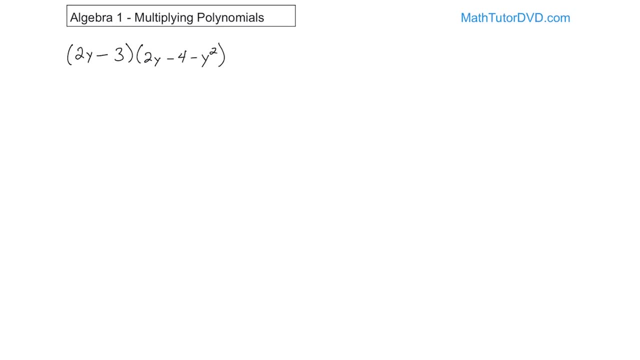 one than some of the other ones is that inside of here normally you want to write a polynomial like this with the highest power in front, So it'd be like negative y squared plus 2y minus 4.. But this one's written backwards with the. 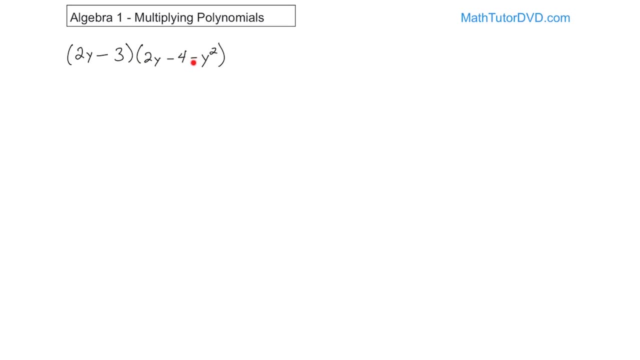 y squared at the end. I guess I'm doing it to show you that it doesn't matter. It doesn't matter the order of the terms. As long as you're taking this and multiplying it times every term, taking this and multiplying it times every term, then you're going to get the right answer. So 2y times 2y. 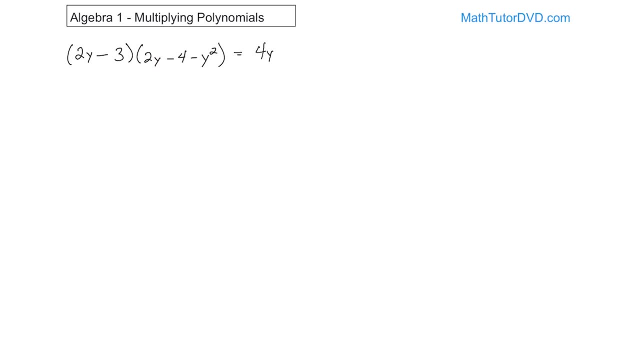 gives you positive 4y And 4, it's not 4y, 4y squared, because we multiply y times y gives us y squared. Then we take this times the next term, times the negative 4.. It's going to give us negative 8y. Then we take this times the last term. don't forget it's negative y. 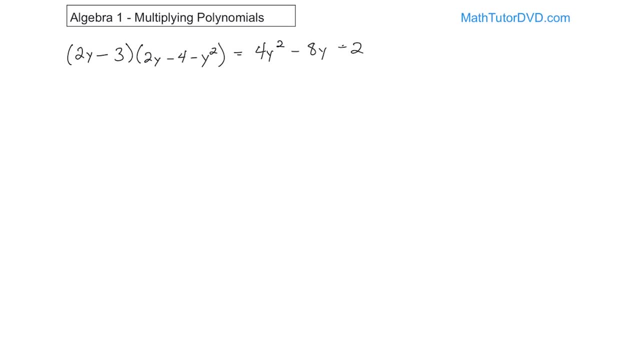 squared, so it's going to be negative 2y to the third power. because we're adding, because we're multiplying y times y squared, so we add the exponents. Now we turn our attention to negative 3 times 2 is negative 6y. 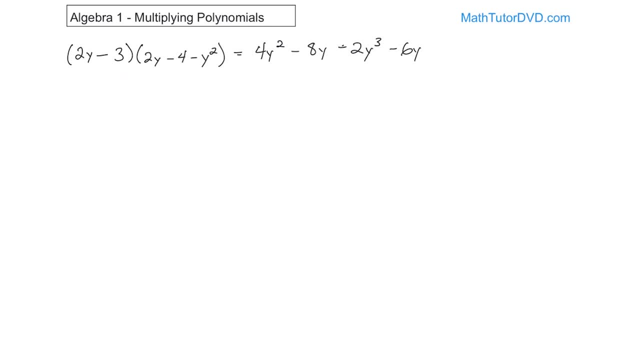 Then negative 3 times negative: 4 is positive 12.. Then negative 3 times negative: y squared is positive 3y squared. Now we do the exact same thing. we collect like terms. We generally want to write the highest powers first, So we look. 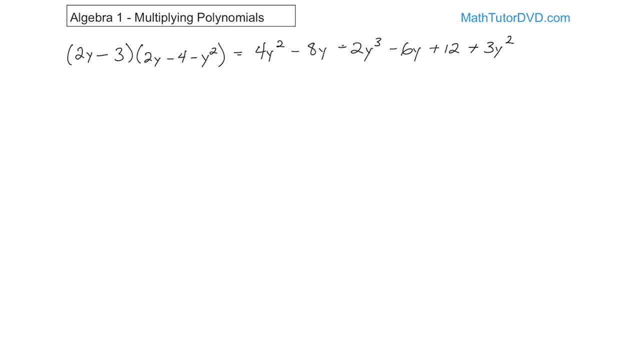 we see we have the 2y cubed here, negative 2y cubed. We don't have any more y cubed so we write it as negative 2y cubed. We write that first. Then we look for any y squares. We have four y squares and we have a 4y squared, But when we put we're 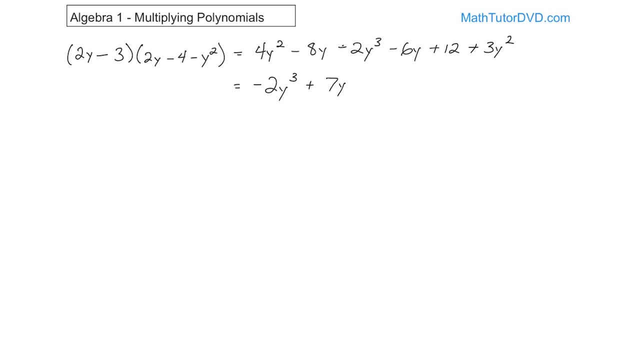 3y squared, so we can add those and make 7y squares. Then we have negative 8y. that's a like term with negative 6y, which is going to give you negative 14y, And then there's only one number. 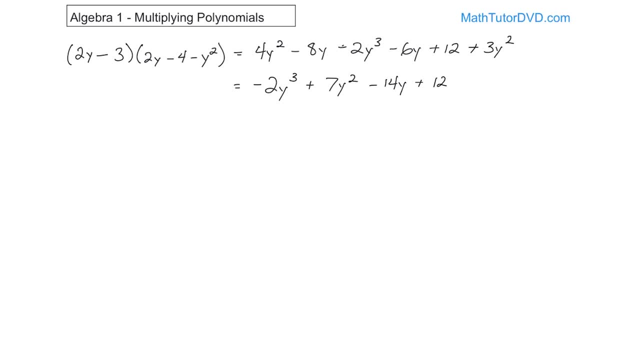 the 12, and he just comes along for the ride. there's nothing to add there. So you get negative 2y cubed plus 7y squared minus 14y plus 12, that's the final answer. And then we're just going to do one last problem. 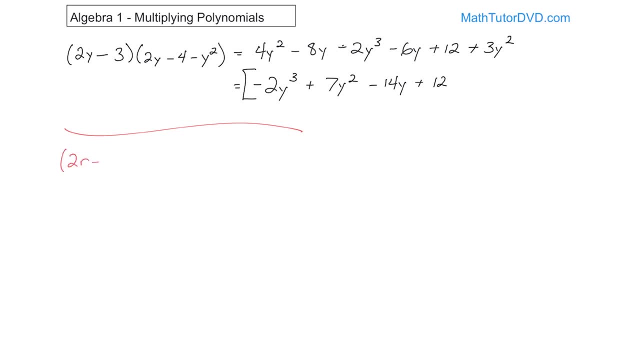 just to give you one more example: 2r minus s s squared plus 4r squared minus 4rs. Now, the only thing interesting about this one is that I have a variable r and I have a variable s, And here I have variable r and s, and here's r and s here. 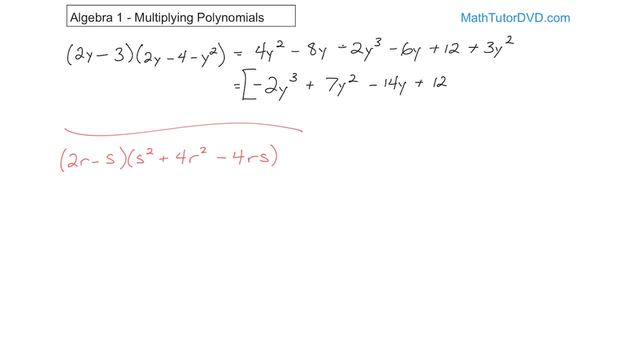 But you're doing exactly the same thing. don't get scared off if you have lots of little variables. All you're going to do is take this, multiply him times each term, adding exponents where you need to, and then you'll take this and go and multiply him. 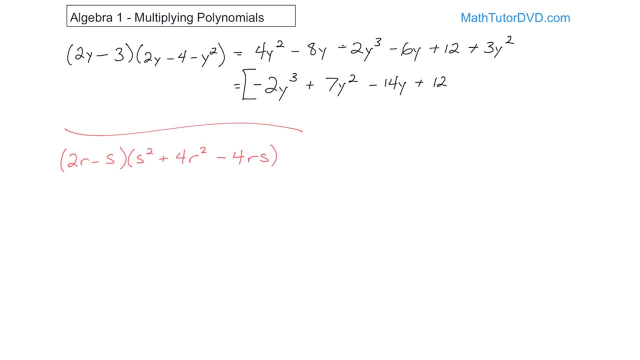 times each term. So 2r times s squared is just going to be 2rs squared. You can't add exponents or anything, because these are two completely different variables, so you just have to write them as they're being multiplied together. 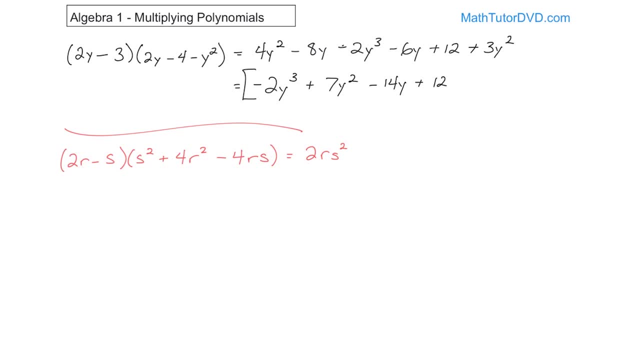 Now you have 2r times 4r squared, which is going to give you: 2 times 4 is 8, and then it'll be r cubed, because here you have an r and an r squared, so you add the exponents. 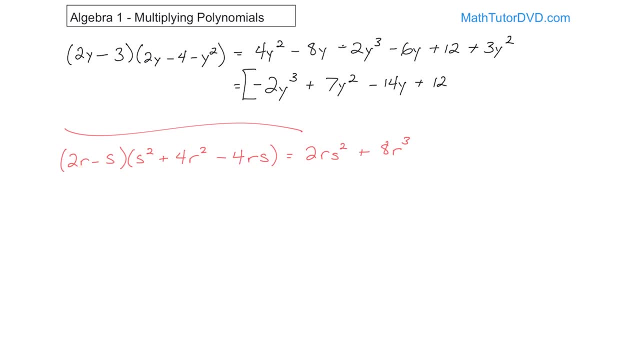 Now this 2r times this last term, 2 times negative 4, is going to give you negative 8, and it's going to be r squared s, because I have r times r, so I add those exponents, but I still have the s. 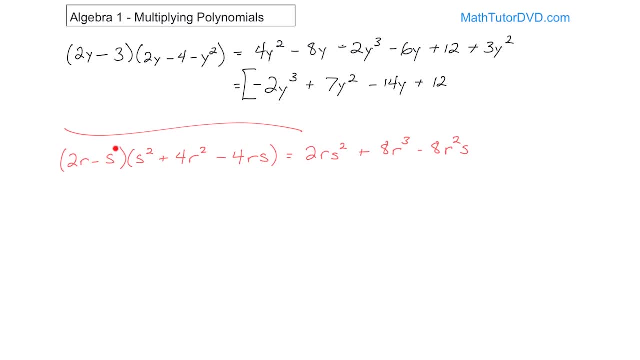 so I have to carry him through. Now I turn my attention to the next guy: Negative s times. this is going to give me negative s cubed adding the exponents. Then I take negative s times, 4r squared it'll be. 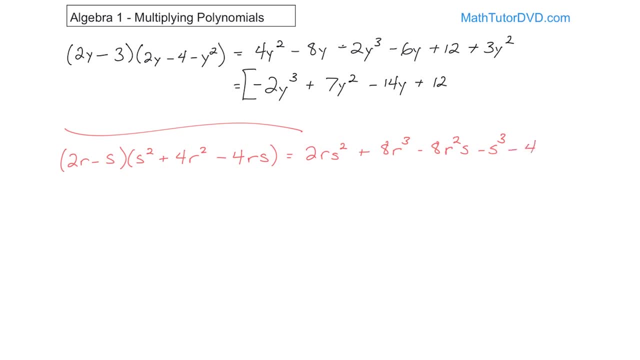 negative 4, and I'll write it in. So I'm going to write this as, just to make it clear, sr squared, because here I have the s and I have the r squared. I can't do much with it, so I just write it down as it's. 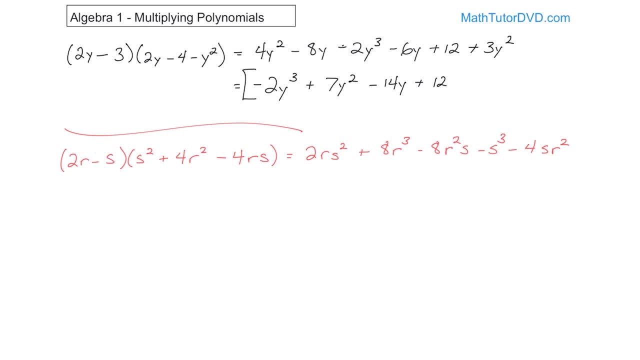 multiplied together, Then the negative s times this negative times. negative gives you positive 4, and then I'll write it as rs squared, because I'm multiplying this times this, so the r is there, and then the s times. the s gives you s. 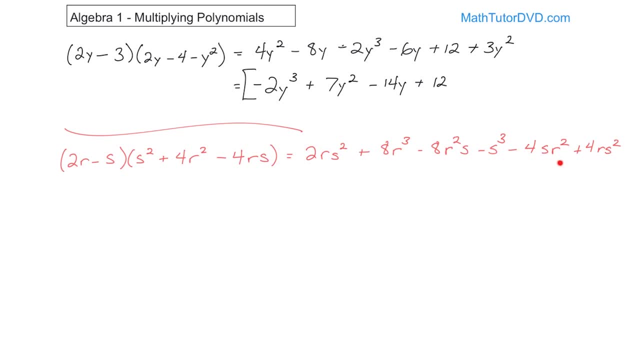 squared right there. So I know that this looks ugly and it is a little bit ugly, but all you have to do now is combine like terms And remember, in the order for something to be a like term, the variables and the exponents have to. 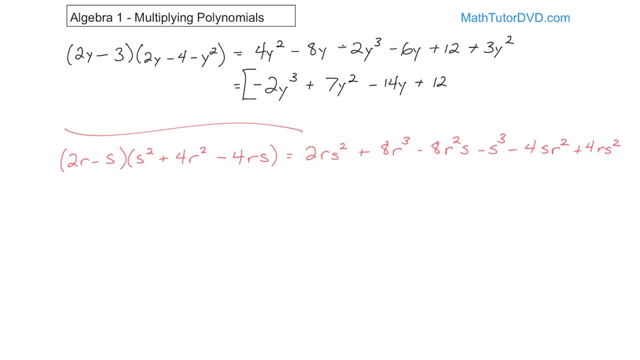 exactly match. That's the only way you can add things together in algebra. So we see that we have an r cubed here. We have to start somewhere. start with the highest power. we see So we have an 8r cubed. 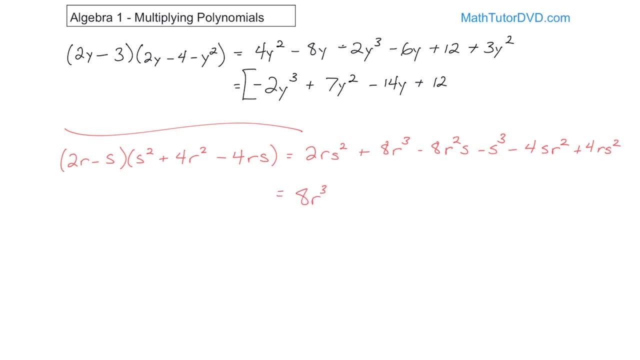 So it'd be 8r cubed, And sometimes it's nice to go ahead and put a dot underneath a term if you've already taken care of it, so that you don't accidentally add things two times. Then we start scanning around for the next, you know. 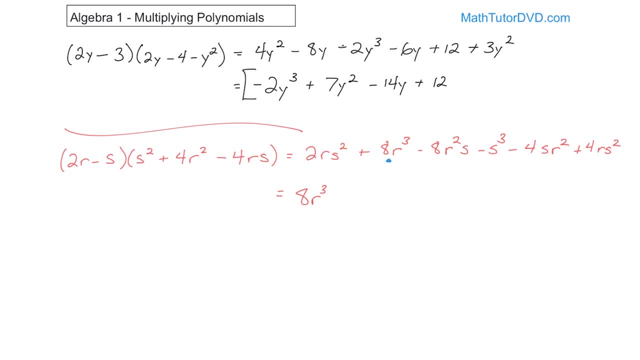 there's lots of different ways you can write it, but the next highest power. But in this case we have next door. we have negative 8r squared s. Let's go ahead and write that next. And so we have negative 8r squared s. 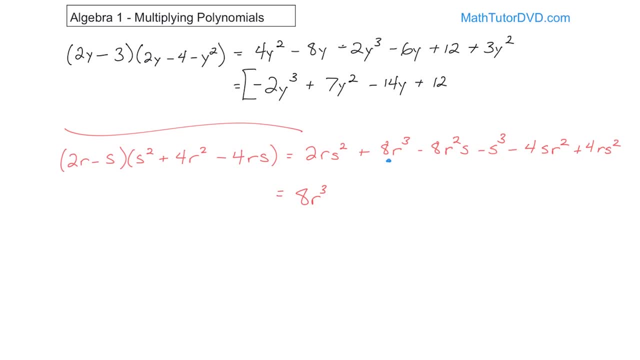 Look at this: We have 4rs squared right here And here we have sr squared. Now don't get confused: here This is r squared s and this is sr squared, But they're multiplied. these are multiplied together, so s times r squared is the exact same thing as r squared times. 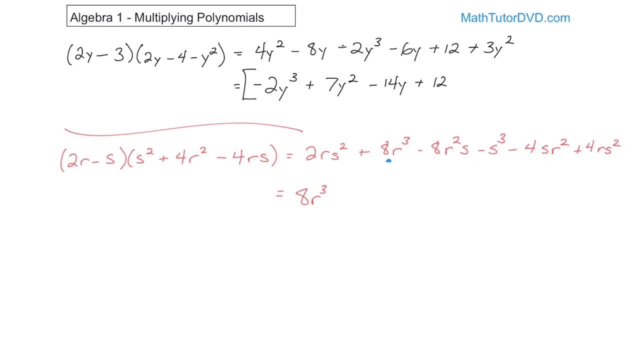 s. So even though these look different, they're actually the same term. So the way that you would write that is negative 8 plus negative 4, gives you negative 12r squared s, Because what I did is I'm adding this term to this term. 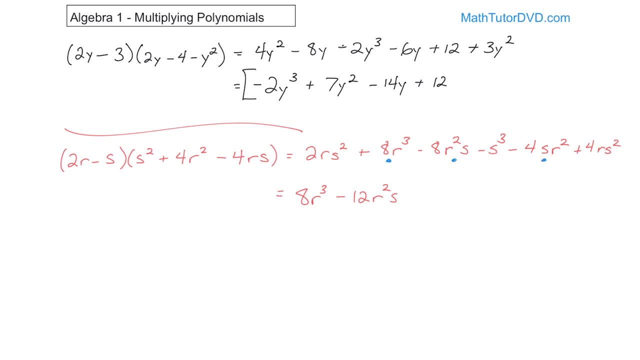 And they are like terms, because I could have written this as r squared s and it would exactly match that. Now this one's completely different. This one's a match with this one over here, So it kind of depends on how you write it down when. 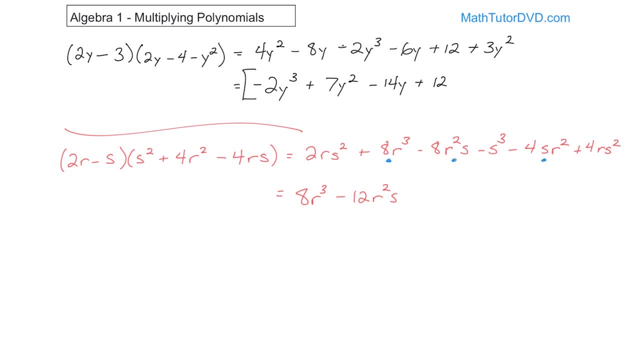 you're doing the multiplication, But when you're combining terms you need to make sure and look and see and make sure that these are right. So here you have 4, and then you have 2.. So then you have 6.. 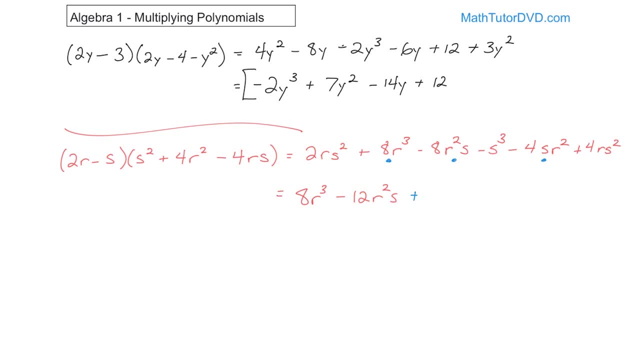 Let's go ahead and take that away. We'll have 6 rs squared like that, And that takes care of this term along with this term. There's only one term left, so you have negative s cubed, Alright. so this is the final answer and that's that last term, right there.